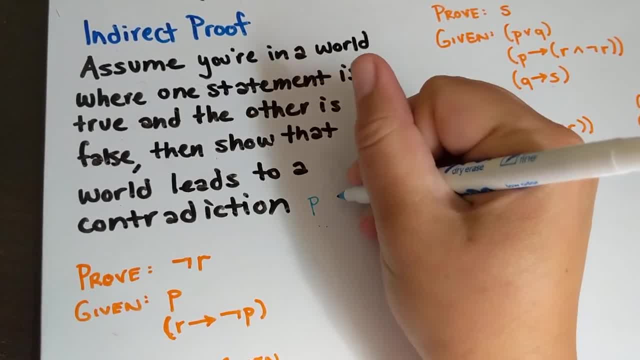 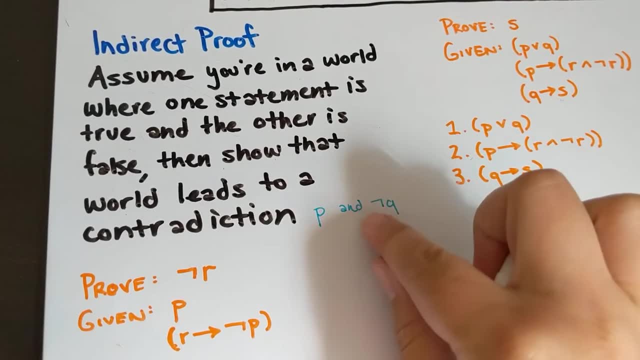 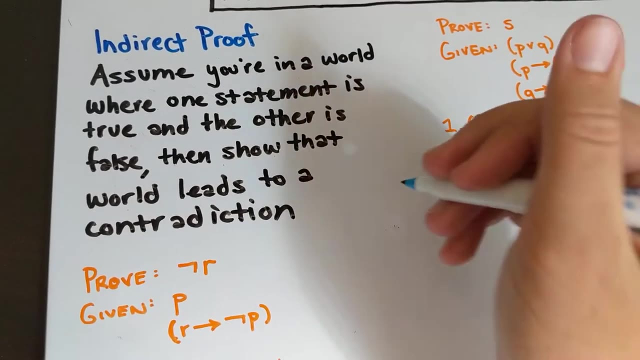 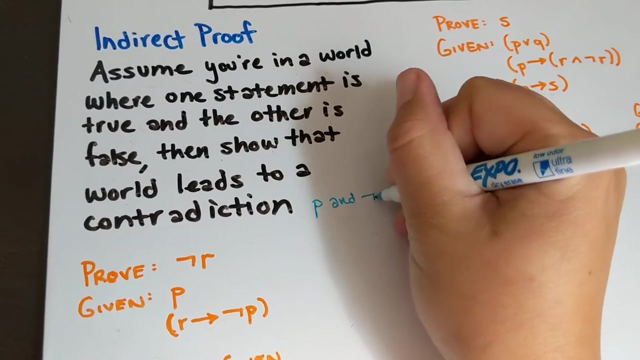 both P is true and not Q is true, right? You should be able to have such a world if they really are not logically equivalent, right? But if they are logically equivalent, then it should be impossible to have a world where P and not Q. That should be impossible, right, And so you can. 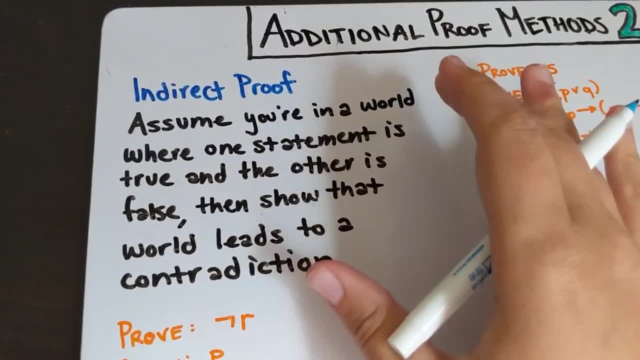 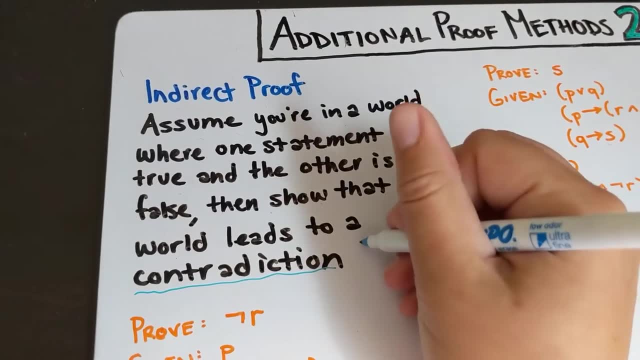 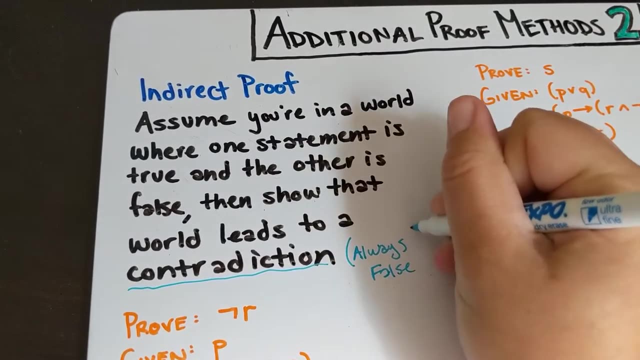 create a fake world in which part of your statement, one of your two statements, is true and the other statement is false, and if that leads to a contradiction- and by contradiction, remember, we're referring to always false right? so if that leads to a statement, that is just false. 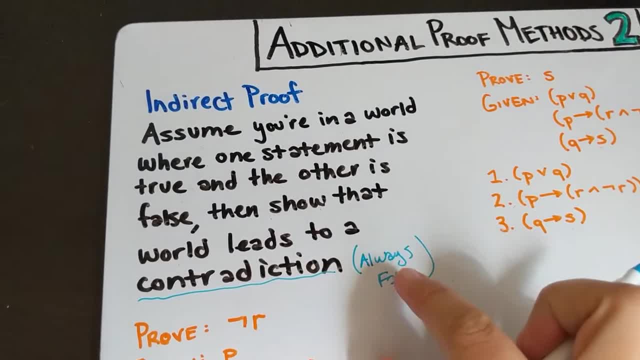 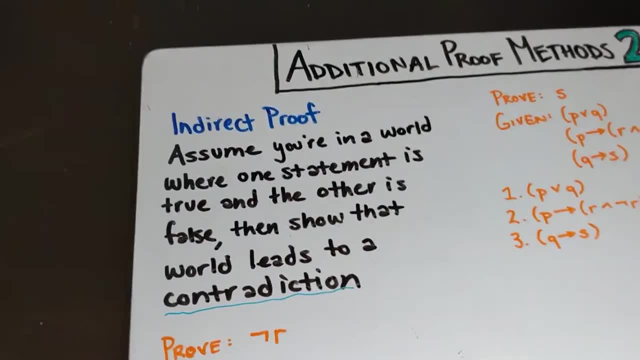 always false, it's always impossible. then you know that you have two statements that are logically equivalent, right, And so you have done your proof. So let's do an example of this. The first example, again, is going to be one of the ones from the book, and we're going to step. 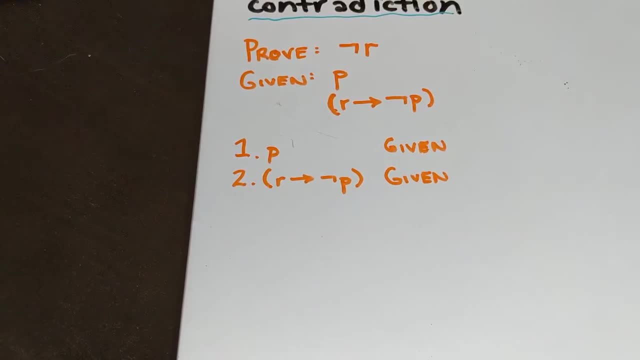 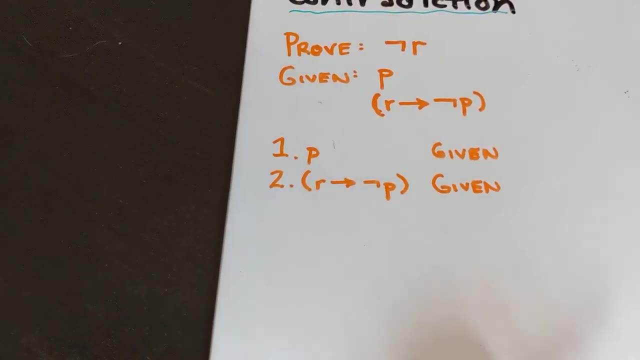 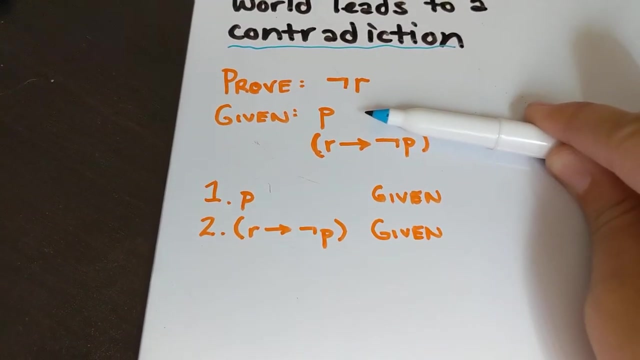 through it step by step, to make sure you understood what was going on when you read it, And then we'll do a statement. that we'll do an example. that was not in the book and is a little more complicated. So we are going to try to prove that not R is the case, given that P is true and R implies not P. 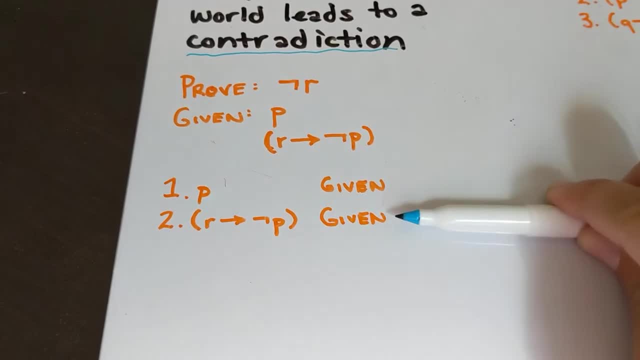 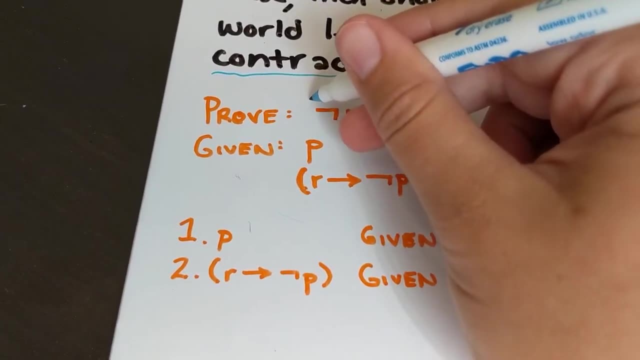 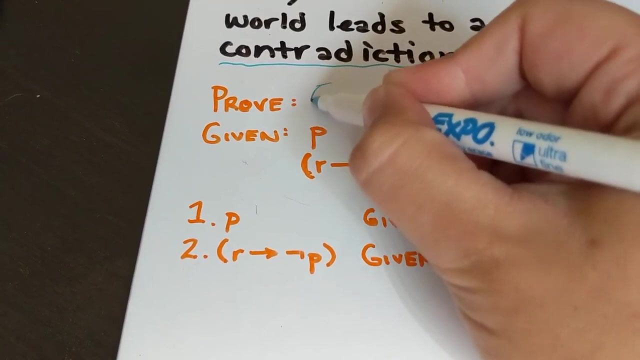 right. So we're going to try to do this proof. So the first step: again, we give our givens as steps one and two, and then we're going to enter our world in which one of these two statements right, So one of these statements is true or is false. So we're going to say that this statement. 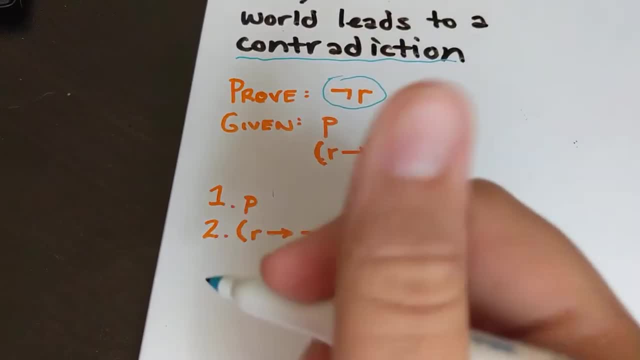 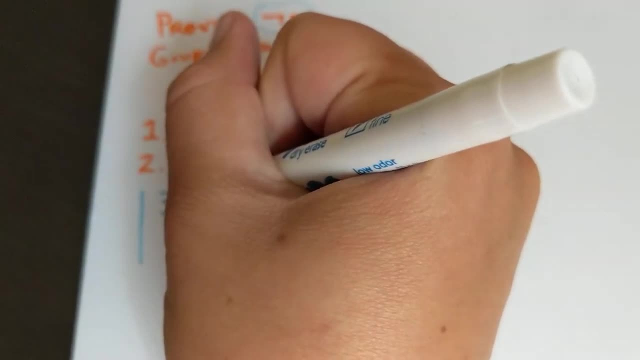 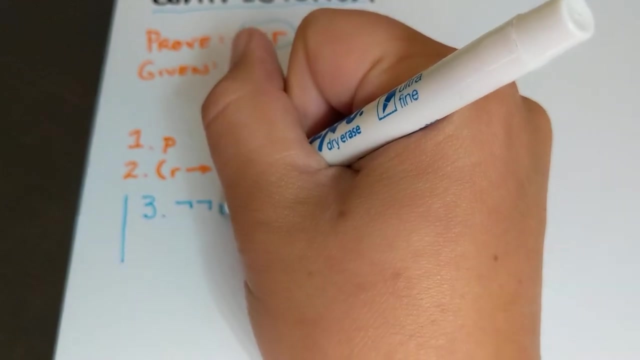 is false In a world where these are true, right? So what do we? what do we do to say that that statement is false? right, We're entering another world, so we have to put our line here. right, This statement is going to be false. so we say not, not R, And this is our auxiliary premise. 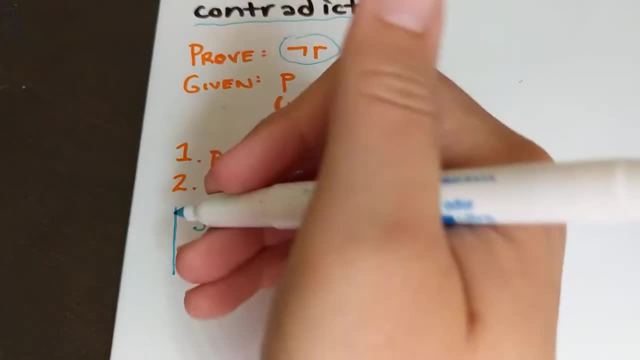 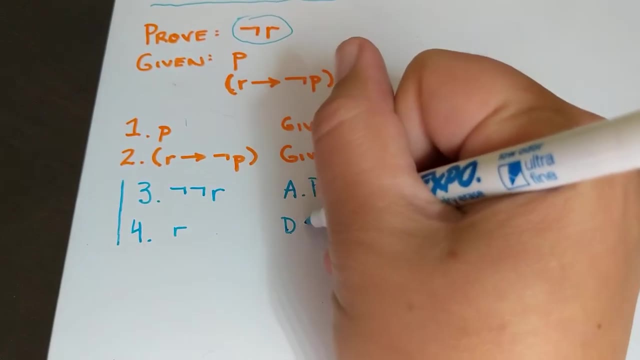 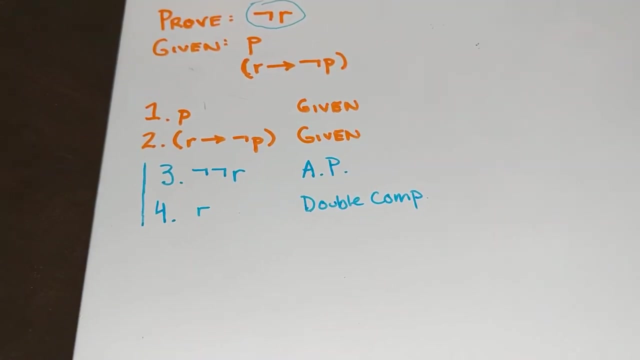 again, This is what we call this. this is an auxiliary premise, And from that we can simplify this down to R using the double complement rule, And once we've done the double complement rule, we can then go back up and look at this right? So 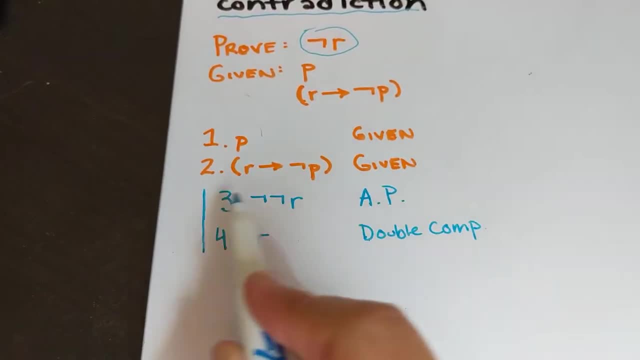 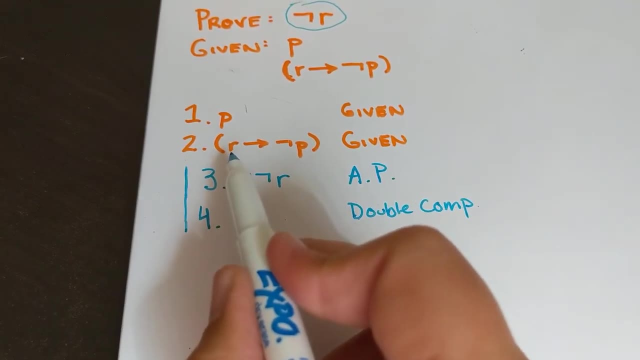 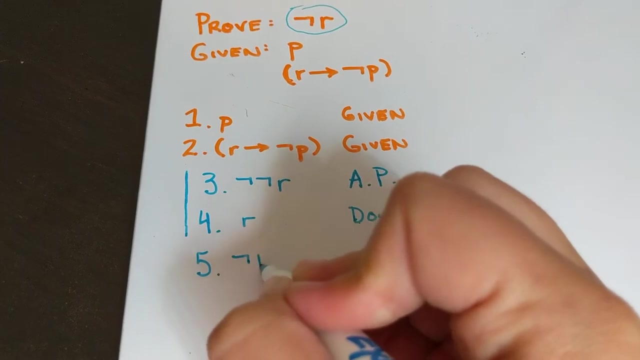 we are still in a world where these two things are true, right. So, even though we're entering a world where this one's false, we're still in a world where these things are true, And so we can still do modus ponens, using this and this, to say that not P is true, And so we can then go back up and 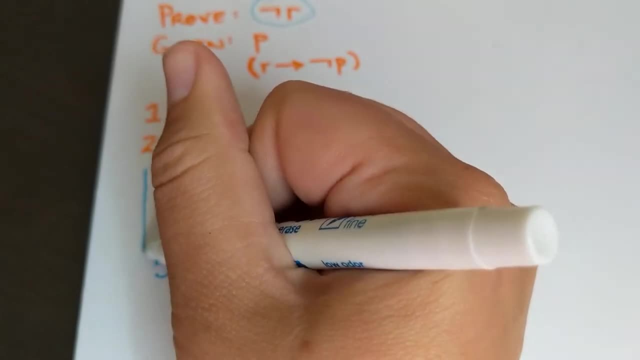 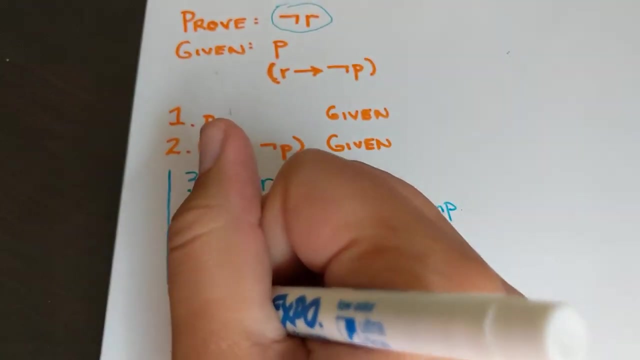 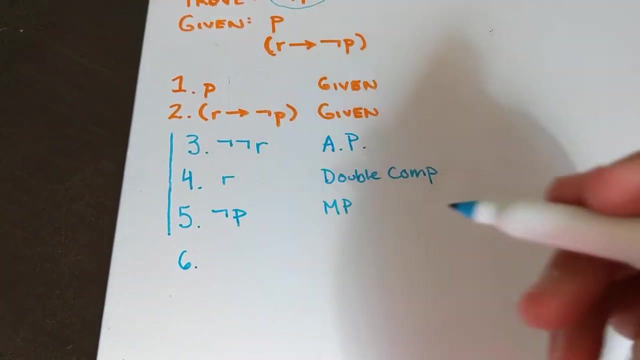 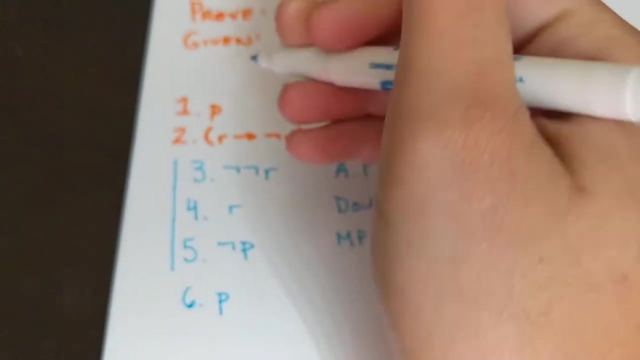 do modus ponens right, Which means that we are also in a world that, in this fake world where not R is false right, We can say that R is true or that P. sorry, that P is true based on this: 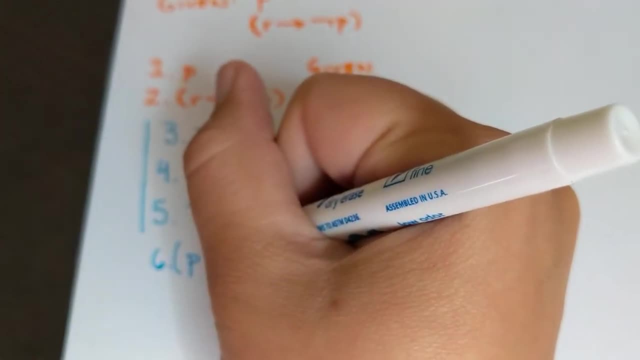 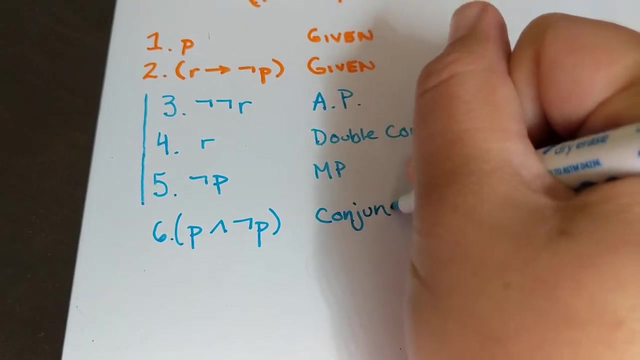 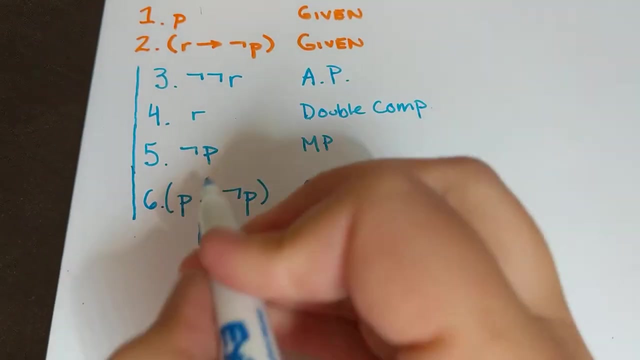 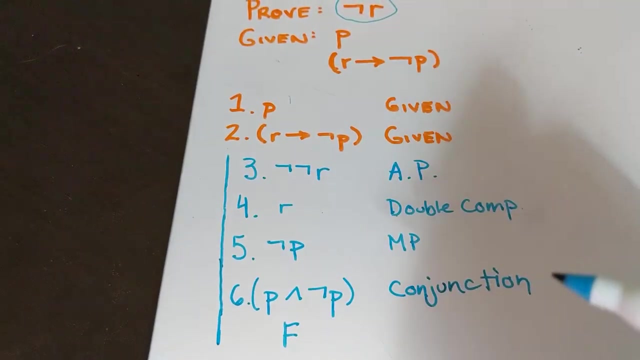 right. Based on step one, we can say that P is true And not P is true, And this is by conjunction, And this is our contradiction, because remember that this is always false, This statement is always false, And so we found our contradiction, which proves that. 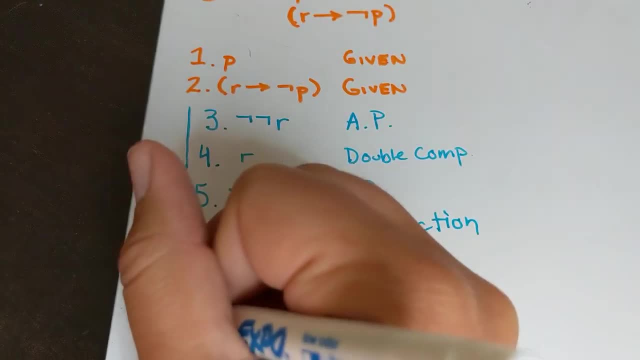 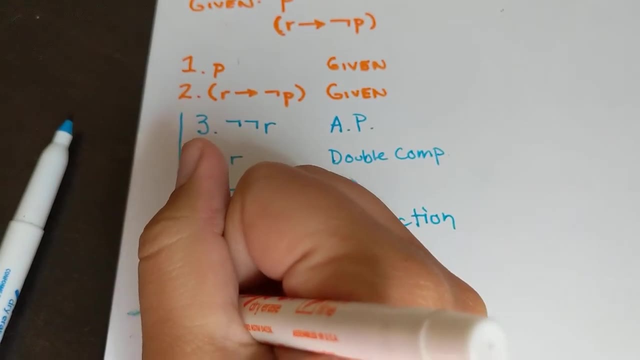 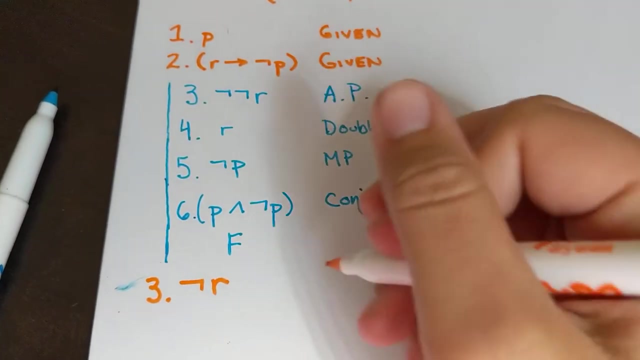 that not R has to be true in this world. Oops, Oh, there are colors here. All right, So it proves that we are in a world where not R has to be true. otherwise, the world is a contradiction, right? Otherwise, the world is impossible, And we've proved this using an indirect proof. 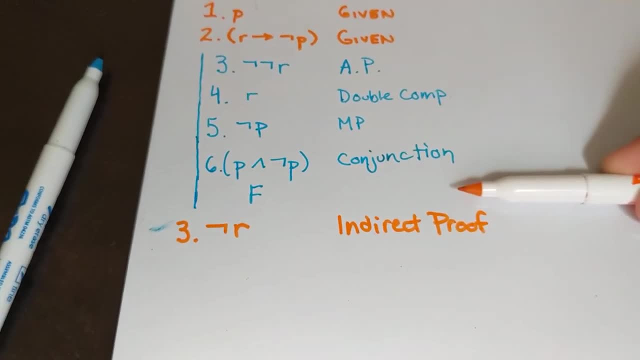 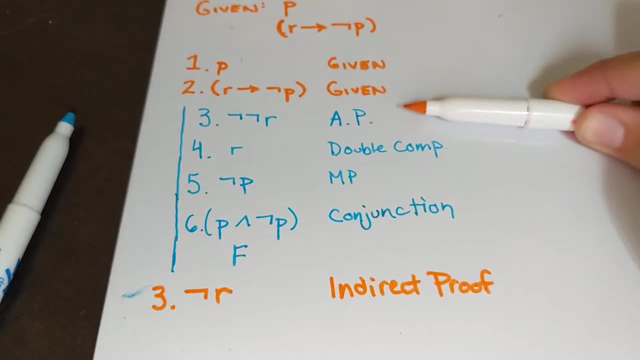 Right, so we cannot have a world like the world in blue, And since we cannot have a world like that, then we have, since this was our only thing setting up this alternate universe. right, this was the only thing that we used to set up the alternate universe we. 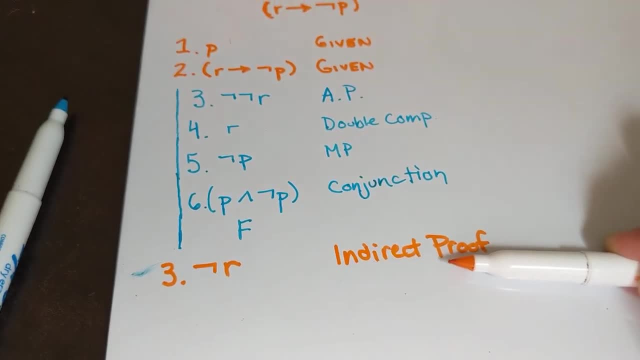 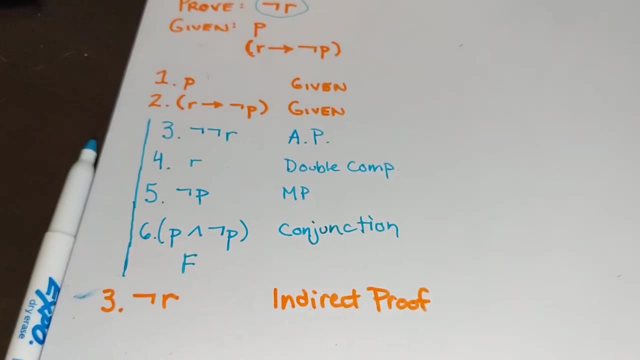 can conclude that this must be wrong in the real universe right, which is the universe in which these are true. So that is how an indirect proof works. Now we're going to do a sort of multi-step indirect proof where we have to do an. 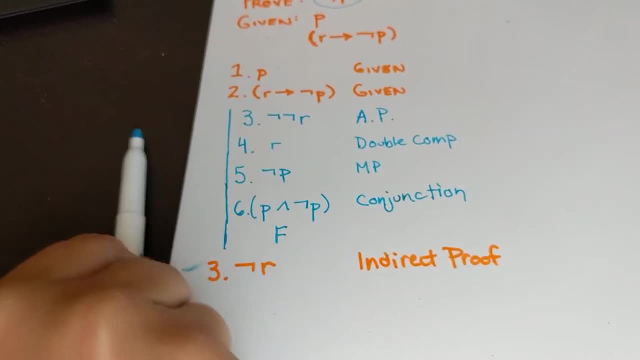 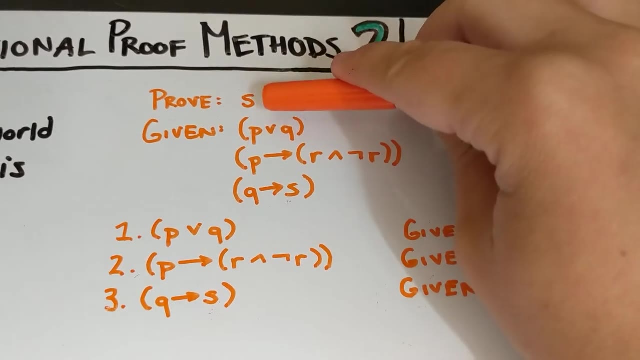 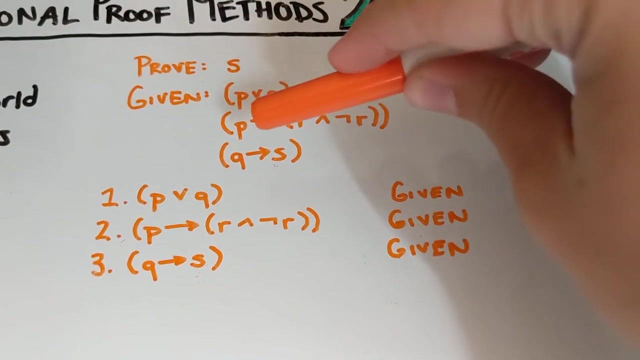 indirect proof halfway through and that's not going to be our whole proof. All right, so we are gonna try to prove that S is true, given that P or Q, P implies R and not R and Q implies S, right. so these are very weird statements. 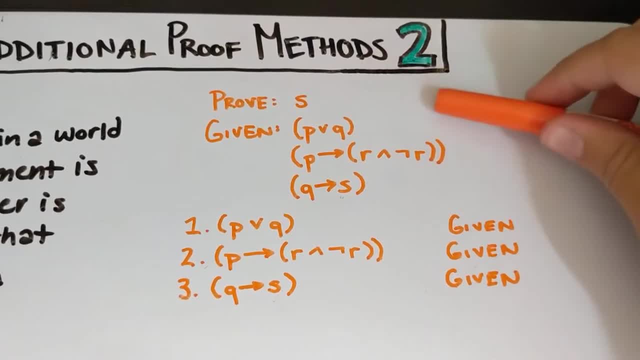 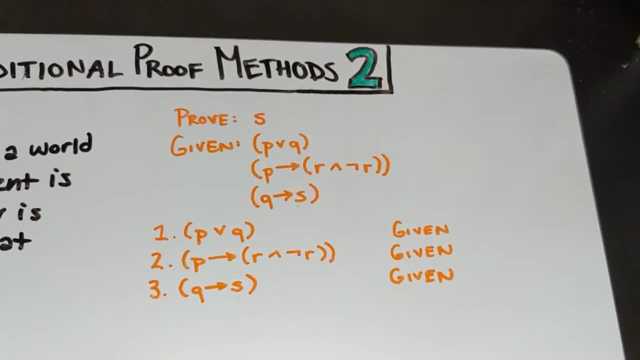 but? but we're gonna use these given statements in order to prove S All right. so the first thing that we do is that we put our given statements down Now, for reasons that we'll get to in a second. We're also going to add a step where we 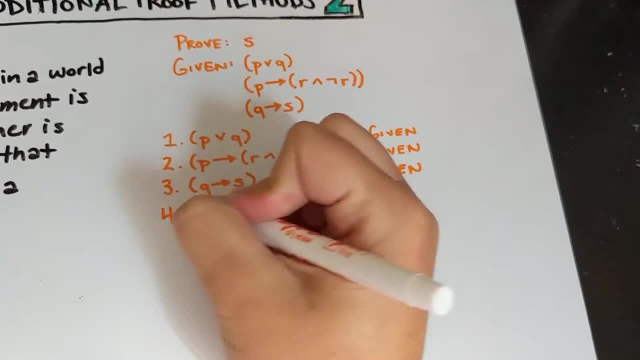 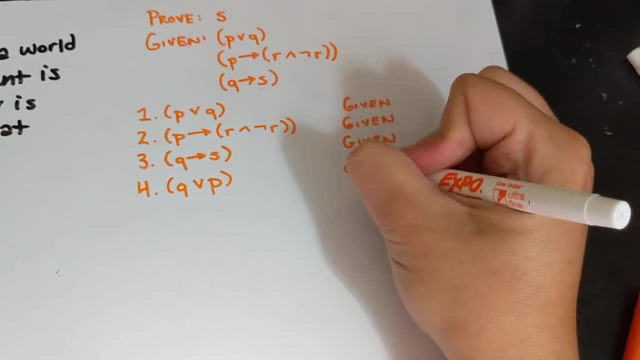 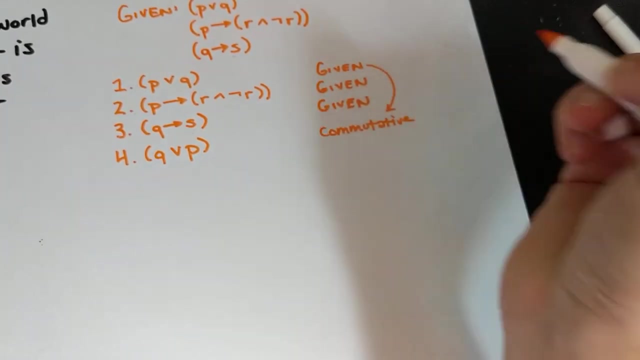 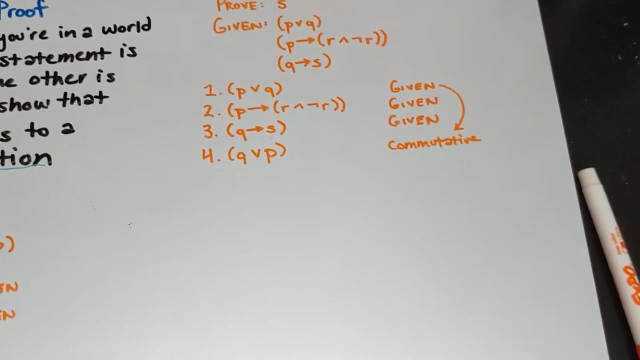 change the order of two of these things so that it says Q or P instead of P or Q, and that's from this rule. I'm using that rule to do that, Alright, so that's just something that we're going to do really quickly. It'll be clear in a second why. 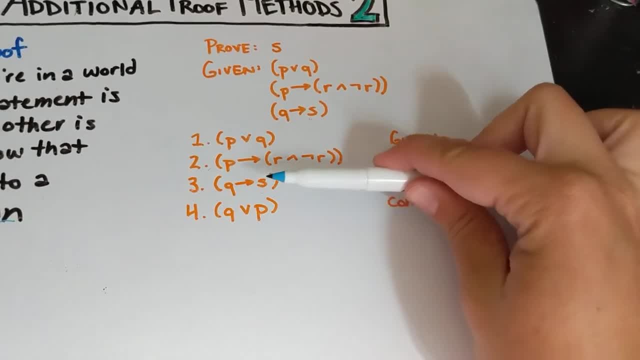 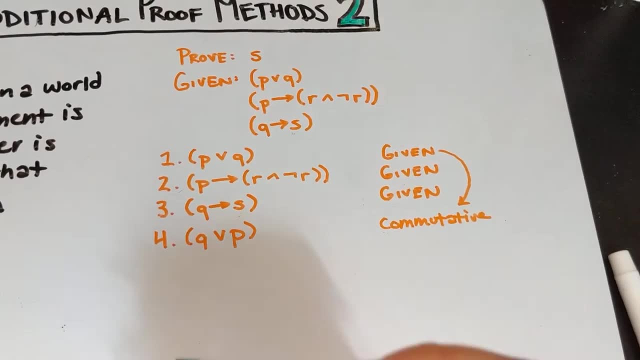 we have to do that. You could. you know, if you had gone on to just immediately enter our indirect proof world, that would have been fine. You would just have to go back and add this step later, when we get to a point where we need it. Alright, 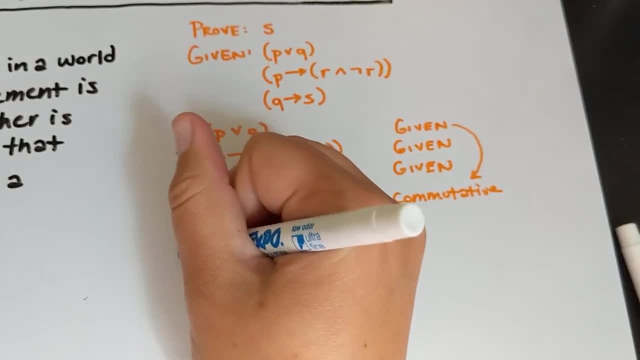 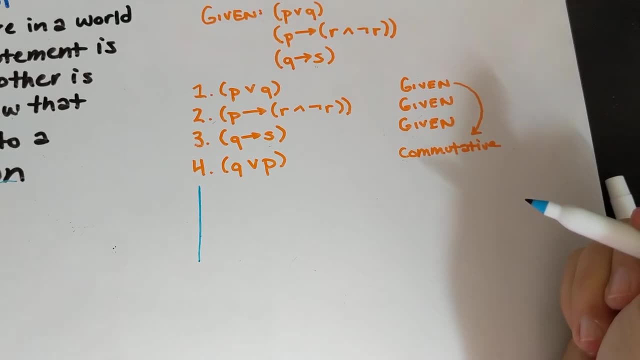 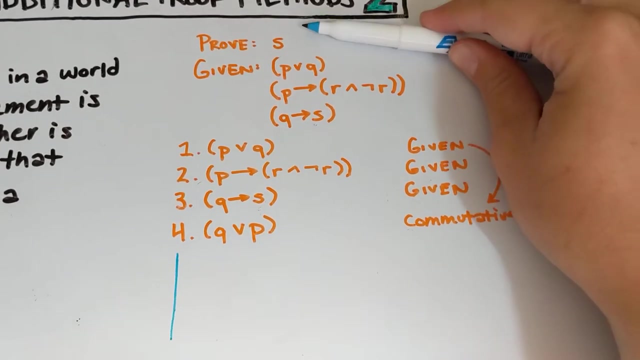 so now we are entering our hypothetical world in which something that we're trying to prove is logically equivalent is not logically equivalent. Now, we might want to. we might be tempted to just immediately say: well, all we're trying to prove is this right, but we're. 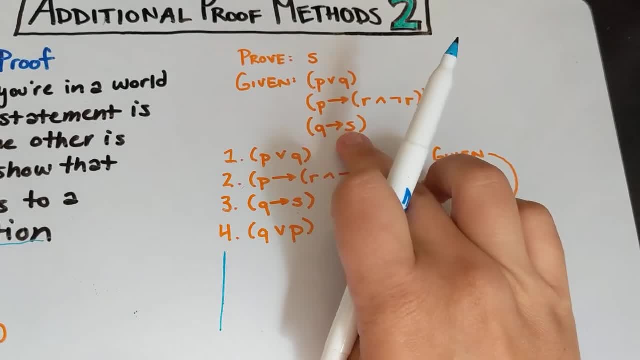 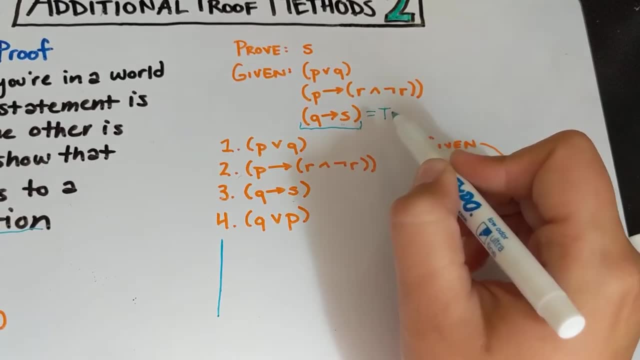 actually going to try to prove an intermediate step, right? so if we want to prove this, since we know that this statement here, this Q-then-S statement, is true, all we have to prove is Q, right? so once we know that Q is true, then we'll know that S is true. So what? 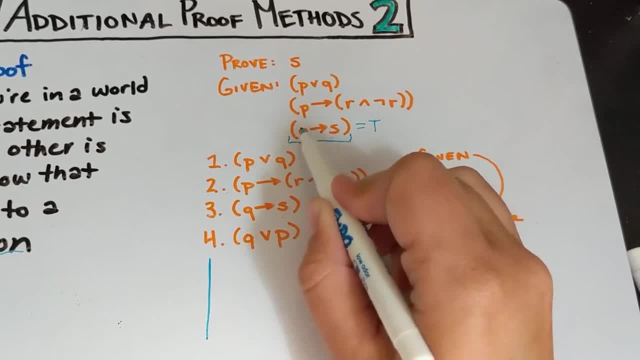 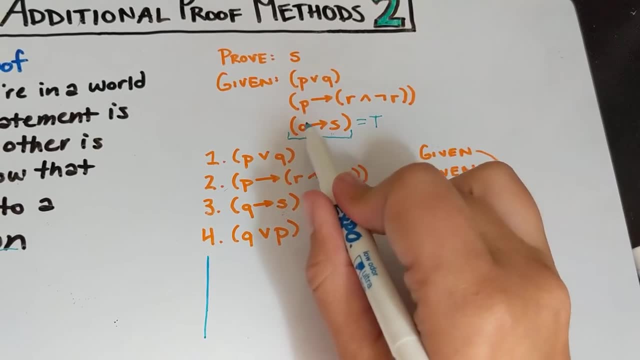 we're going to try to do right now is use an indirect proof to prove that Q has to be true. So this is a little bit weird-seeming, but we're going to prove that Q is true before we and then, just at the end, that'll prove for. 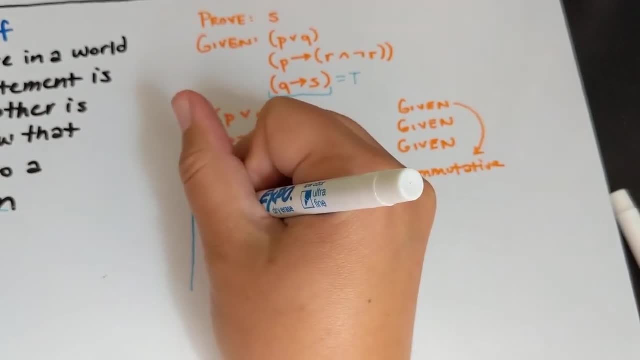 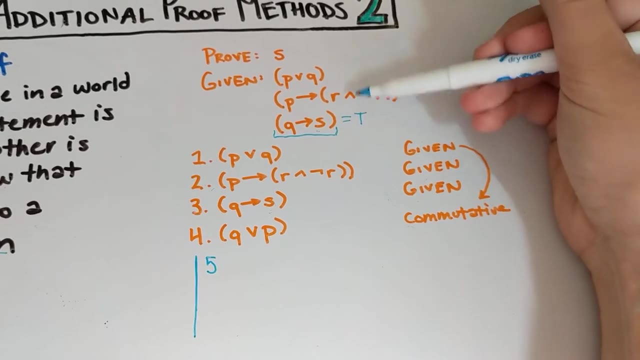 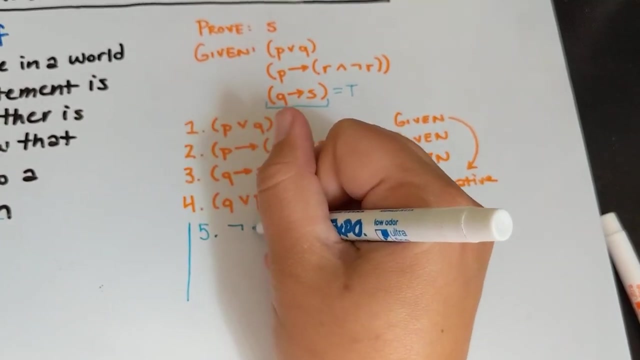 us that S is true. So, since we're doing an indirect proof and we want to prove that, given these statements, given these three statements, Q has to be true, Q has to be in our model, we are going to assume that not Q is true, right? So that's what we're going to use to set up our alternate. 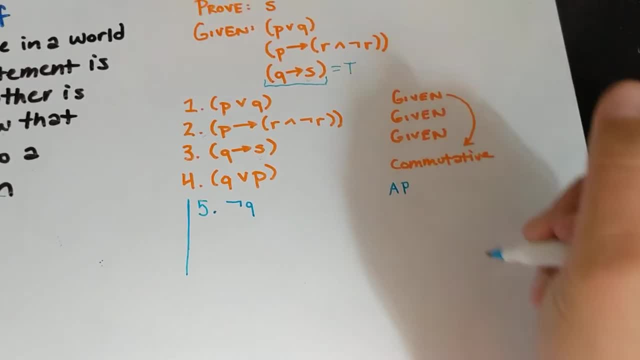 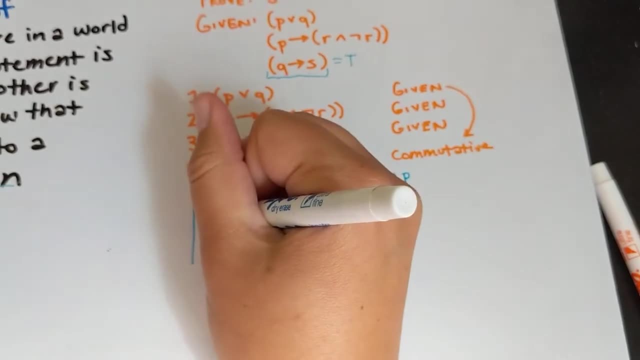 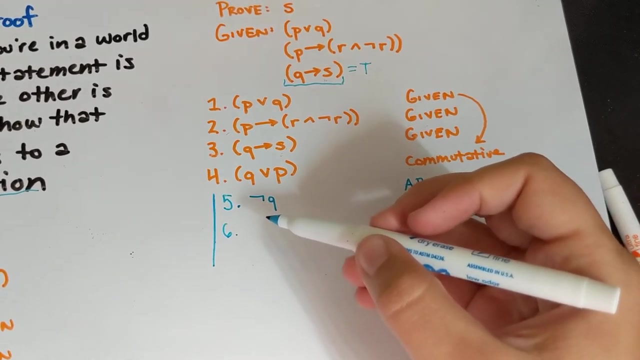 universe using our auxiliary premise, right? So that's. our auxiliary premise is that we're setting up a universe in which not Q is true. Once we know that we can also prove that P, we can prove that P must be true. Now, how can we prove that We use a disjunctive syllogism? 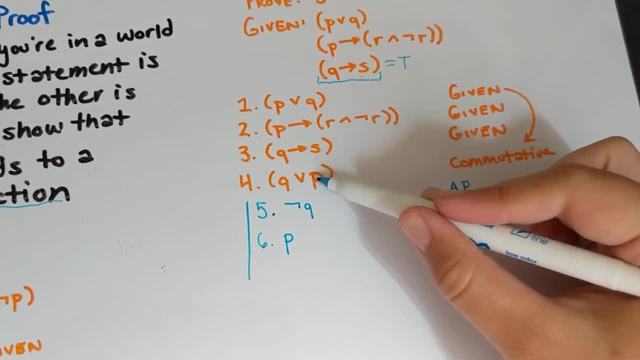 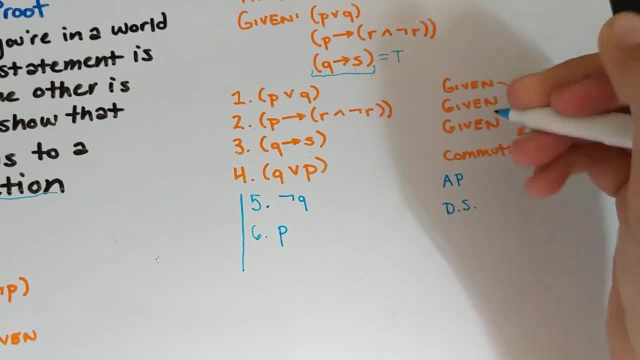 What have we done here? right, So Q or P, and not Q implies P, right? This is the disjunctive syllogism rule. so we're just using these two rules in combination, these two lines in combination with each other. 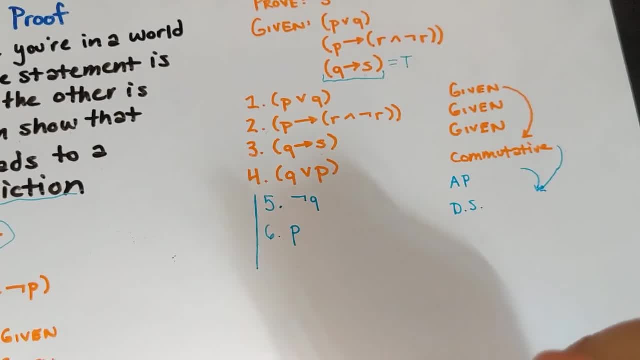 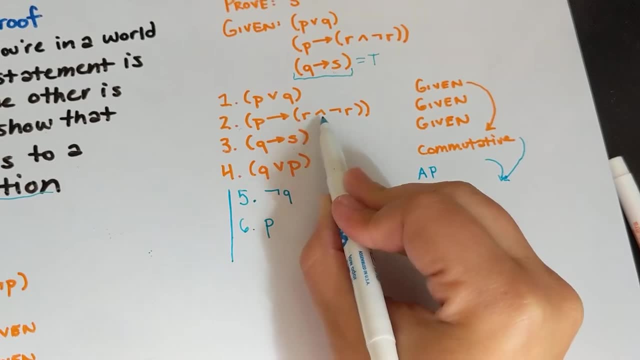 to do a disjunctive syllogism, right? That's what we're doing here. All right, so we've proven that P must be true. If P is true, then we know that R and not R must be true. 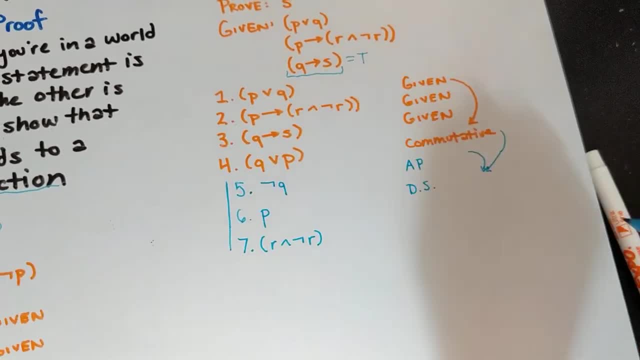 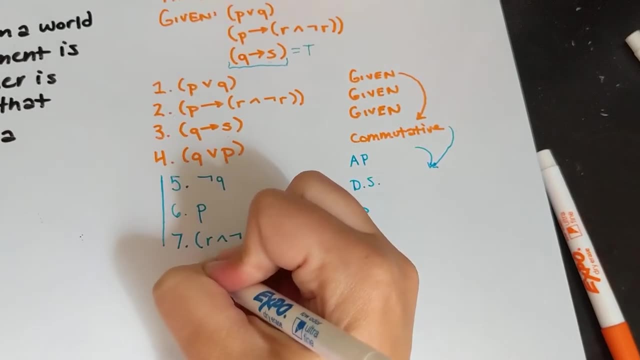 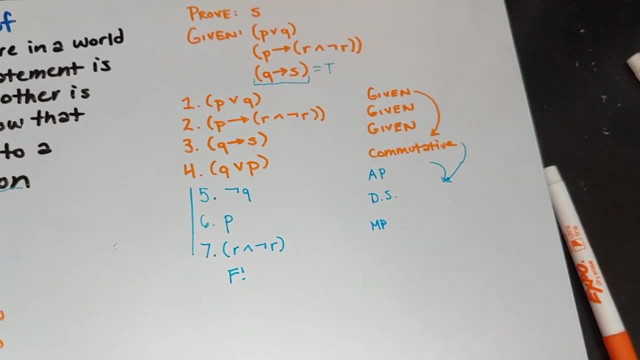 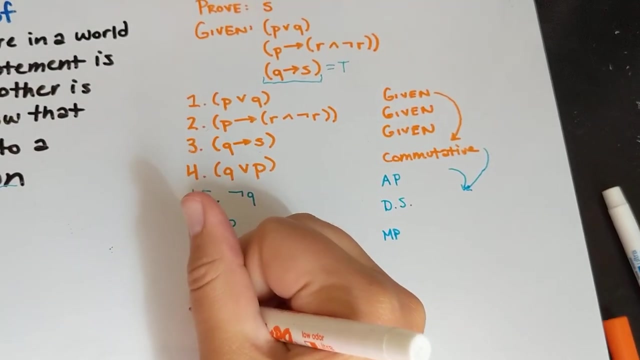 R and and not R by modus ponens. And what is R and not R? It's a contradiction. So there's our contradiction, which tells us that this hypothetical world in which Q is false is impossible right. So we can't have a world in which Q is false. so we conclude that Q is true. 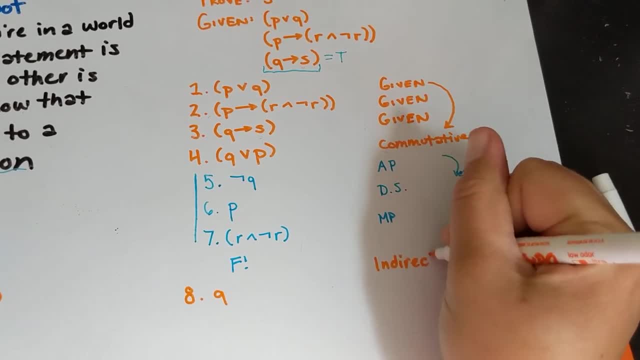 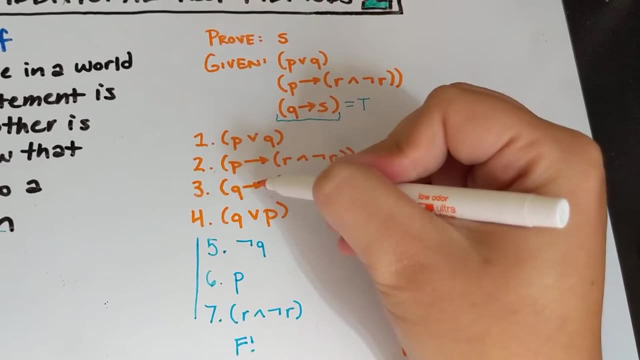 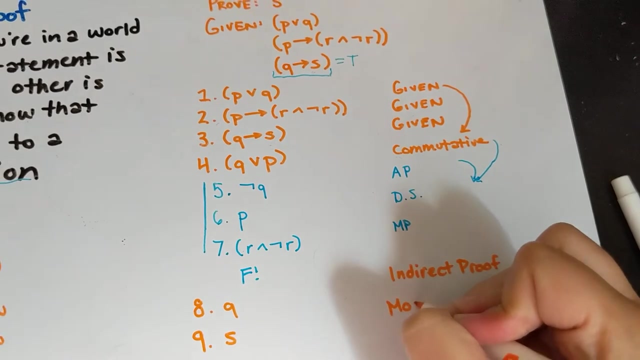 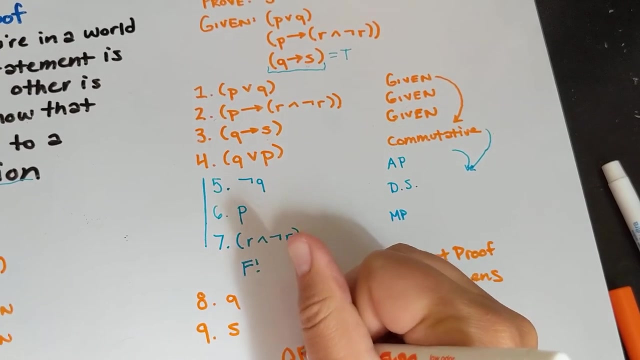 by an indirect proof. And now we can go back up to this, given here that Q implies S, and now that we know that Q is true, we know that S is true by modus ponens And QED. We've done it again, We've proven the thing, and now you guys are all fluent in what an 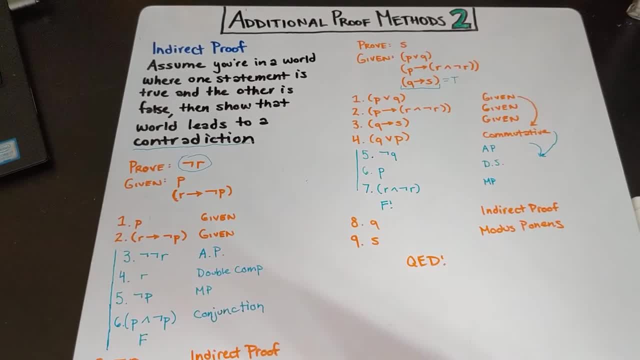 in a way, Indirect proof is right, Right, All right, um. so this has been a video about proof methods.